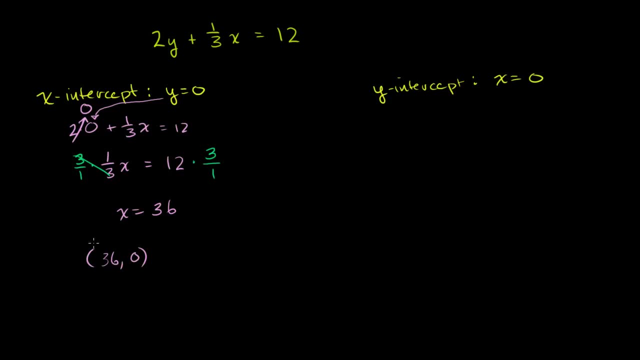 Or the point 36, comma 0 is on the graph of this equation, And this is also the x-intercept. Now let's do the same thing for the y-intercept. So let's set x equal 0. So you get 2y plus 1 third x. 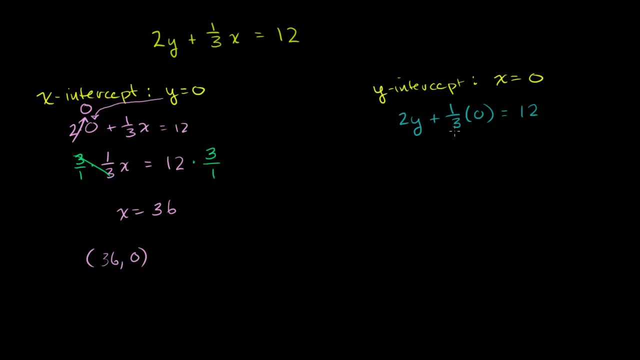 Times 0 is equal to 12.. Once again, anything times 0 is 0. So that's 0. And you're just left with 2y is equal to 12.. Divide both sides by 2 to solve for y. 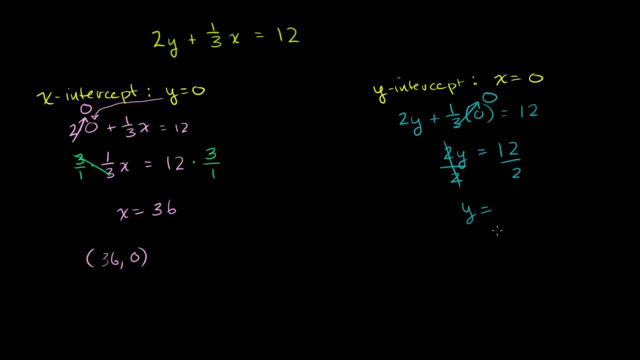 And you're left with: y is equal to 12 over 2 is 6.. So the y-intercept is when x is equal to 0 and y is equal to 6.. So let's plot these two points on a graph. I'll just do a little hand-drawn graph and make it. 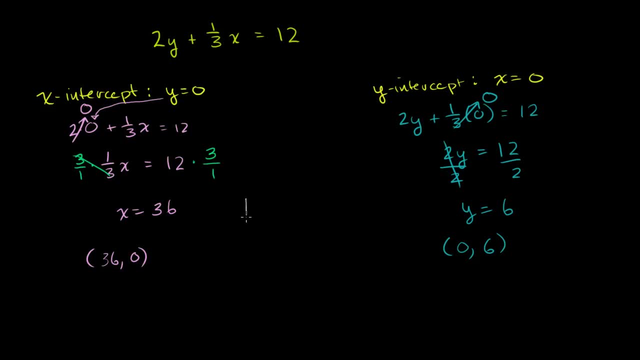 clear what the x and the y-intercepts are. So let me draw: That's my vertical axis And that is my horizontal axis, And we have the point 36 comma 0. So it might be way. So this is the origin, right here. 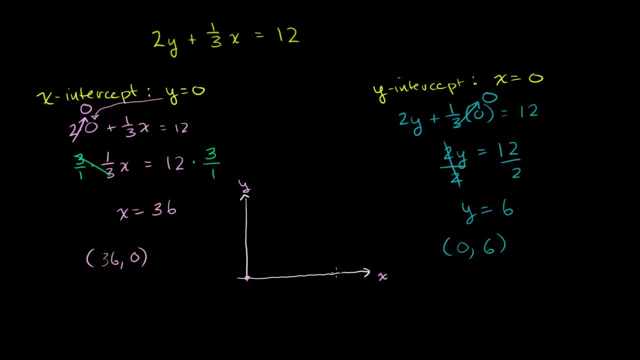 That's the x-axis, That's the y-axis. The point 36 comma 0 might be all the way over here. So that's the point 36 comma 0. And if that's 36, then the point 0, 6 is going to be. 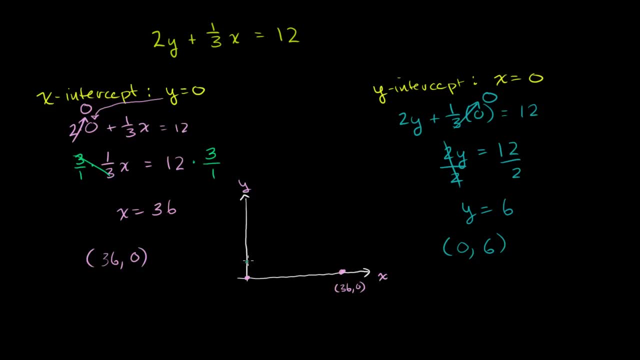 right about 0, 6.. Might be about right about there. So that's the point: 0, 6.. And the line will look like something like this: The line will look something like that, Trying my best to draw a straight line. 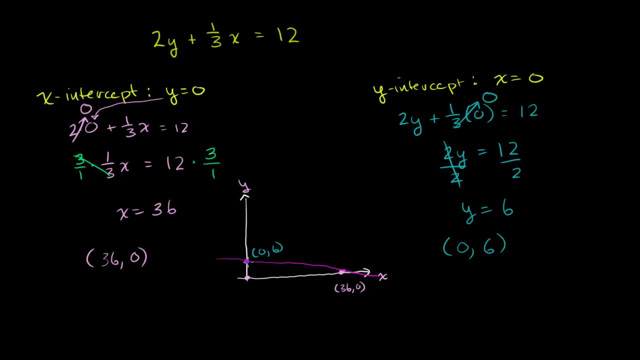